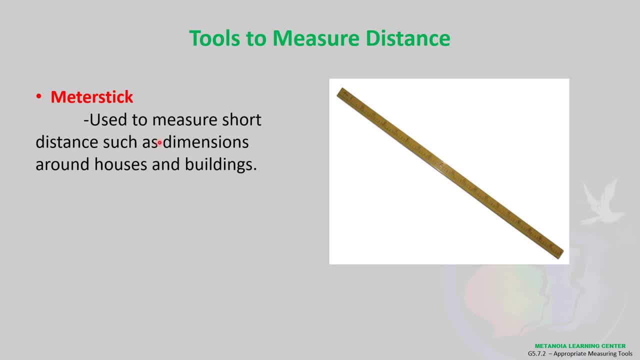 the image that I was able to find online. Okay, Used to measure short distance, such such as dimensions around houses and buildings. So, tulad sa bahayin nyo, What is the perimeter around your house, so you can make use of the units? So this is І wall design, This software, you can use it here. This is the j estructural database You can see on the screen, Okay, and then later, And then later on, I'm going to show you learn more about m 1945, section" and talk it okayak e, if you're interested. gesprochen a alal. 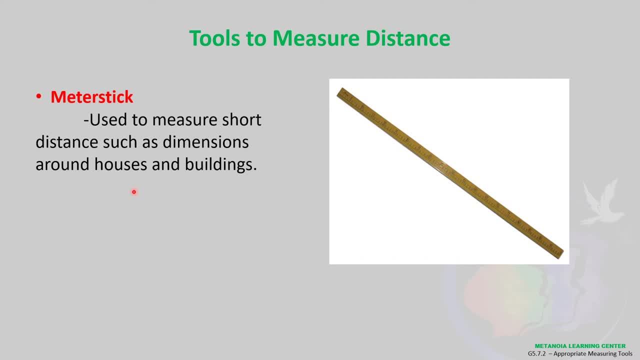 perimeter around your house, so you can make use of the unit of meters to measure the unit around your house or the distance from one point to another as you travel or as you walk from your house to your neighbor or outside your barangay community. okay, also use. it is also used for. 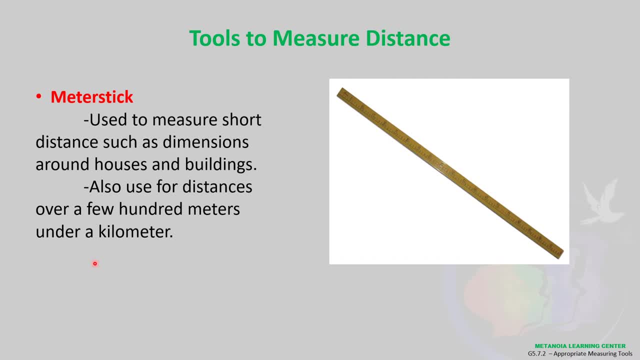 distances over a few hundred meters, under a kilometer. so 100, 1000 meters is equivalent to one kilometer. so that's just a uh basis. so which means if you have a thousand of this, thousand of this, that's equivalent to one kilometer. so let me just also used for: 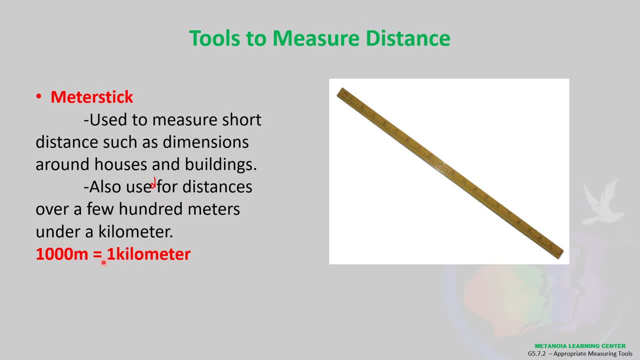 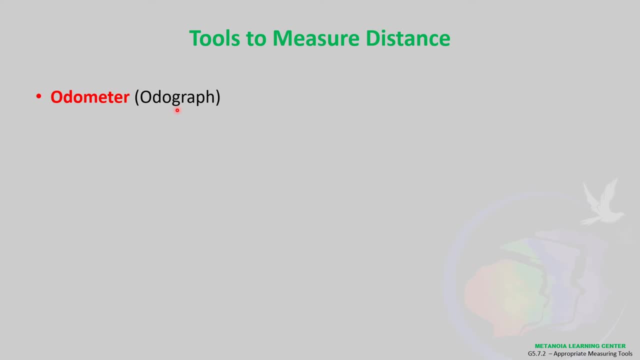 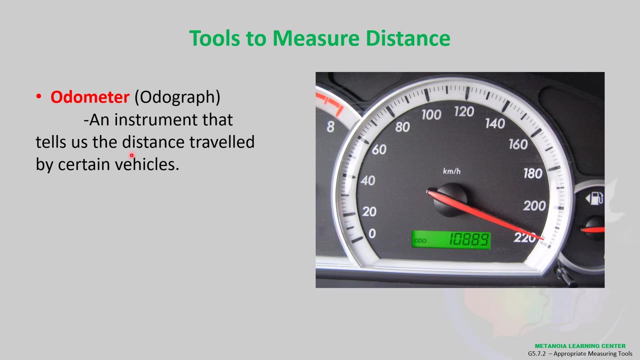 distances over a few hundred meters, under a kilometer. okay, odometer or odograph. so this is an example of another odometer. so this is an example of another odometer. so this is an example of another odometer. just to make it clear, uh, an instrument that tells us the distance traveled by certain vehicles. again, 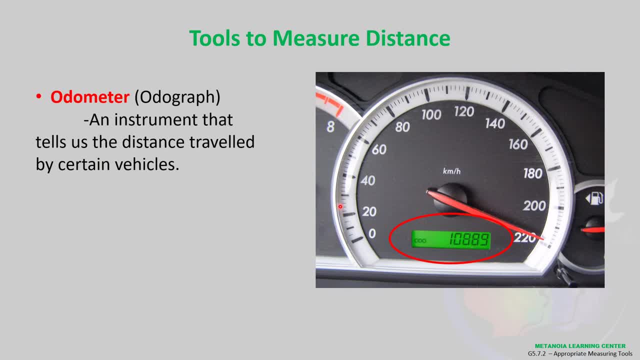 this is the odometer the count here, not this one. okay, because this is called a speedometer. okay, speedometer. speedometer basically measures how fast you are going, while an odometer measures how far you have gone since you bought the car. okay, so, uh, usually you cannot reset that. 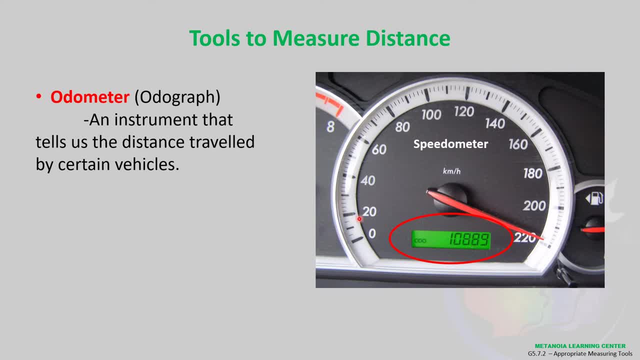 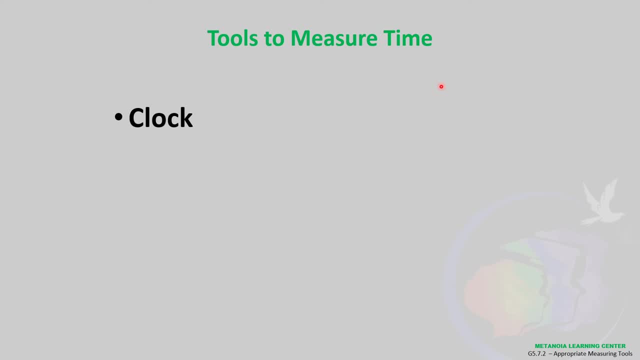 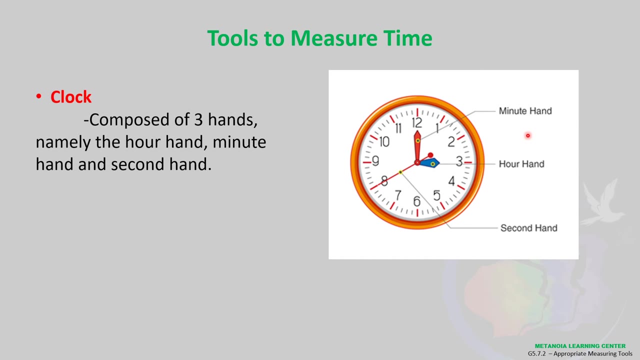 value unless it goes back to zero again, until it reaches its maximum point. okay, so tools to measure time? obviously the clock and the stopwatch. so the clock- you should know by now that we have uh, or a clock- is basically composed of three hands, namely the hour hand, the minute. 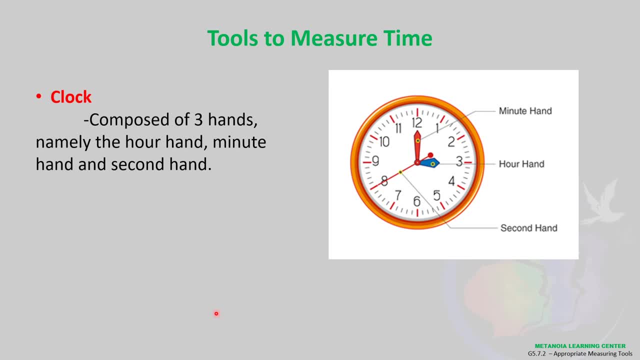 hand and the second hand. you should, of course, know that. so specific hour yan, in other words, no, including the seconds, for example, our uh. for example, you arrived at this certain place at 10 o'clock, that's just by the r some. some people would say: oh yeah, i've been waiting for you. 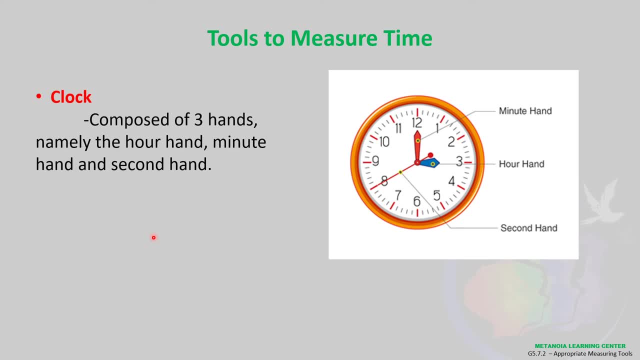 arrived at 10 o'clock. i i was waiting for you since 9: 50.. so that's nine o'clock and 50 minutes, the nine hours and 50 minutes. so meron denisa would tell you that i've been here, uh, since 9: 55. 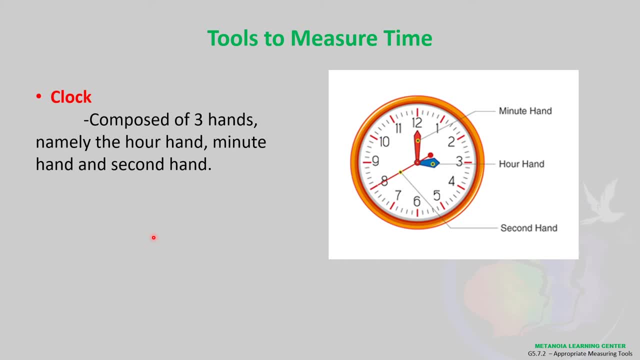 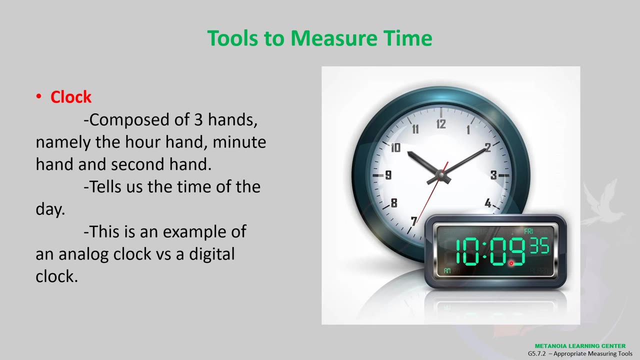 and 30 seconds, so to be specific, but no one says that. of course, tells us the time of the day. okay, that's a very obvious, and this is an example of an analog clock versus a digital clock. so nowadays, mostly we all we already have this, even in our phones- no, which also not tells us the time. 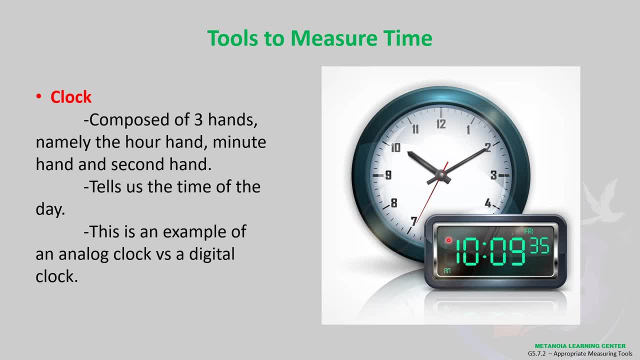 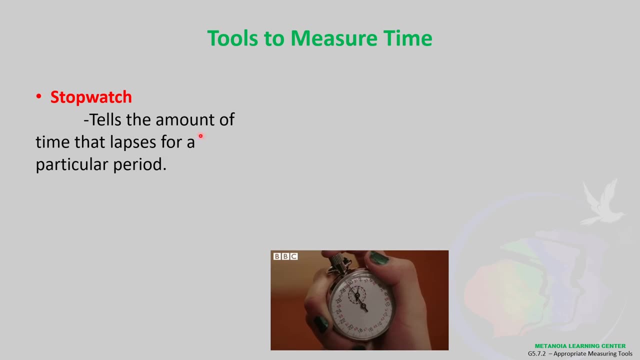 alone, but also uh, the day, and some even have the dates. no, so i don't know exactly. uh, day to day. just like it's a phone, ninja, okay. another one is stopwatch. okay, this is an example of a stat watch, and an analog stopwatch tells the amount of time that lapses for a particular second. 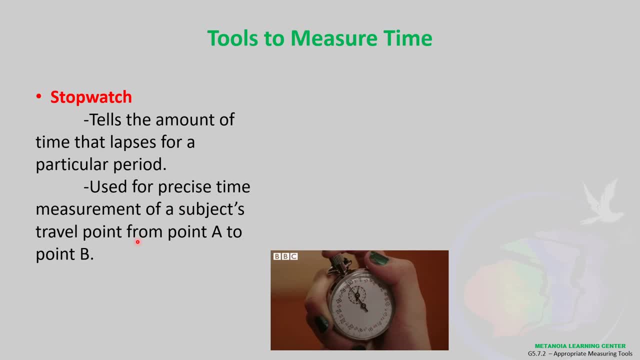 used for precise time measurement of a subject's travel from, uh, point a to point b. okay, why did i subjects travel point? well, well, okay, travel from point a to point b. so, for example, traveling from point a to point b. to be specific, let's say you have two students here, your one is gonna. 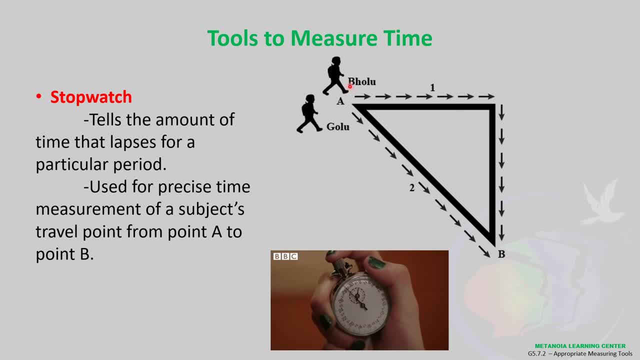 this student- I don't know why the name is Galu and the other one is Balu- might be Indians. am I being racist? I don't know. I hope not. okay, so Balu walks this path. so a person will time how long it will take Balu to reach. 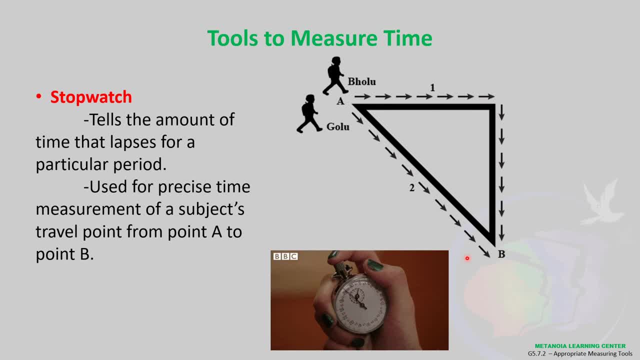 from point A to point B and another one here, point A to point B as well. so obviously this is a shortcut compared to this one around talaga. so anyway, we can tell the difference by minutes and by seconds as well. so that's what's good when you're using a stopwatch. 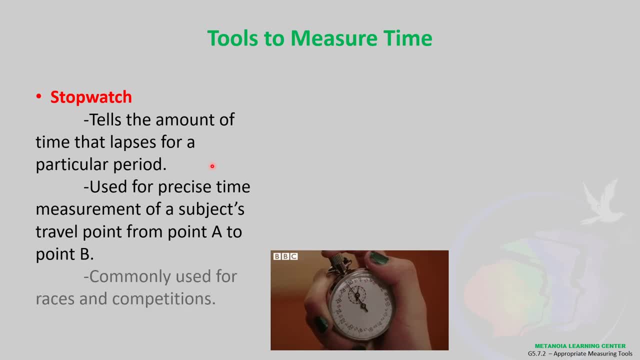 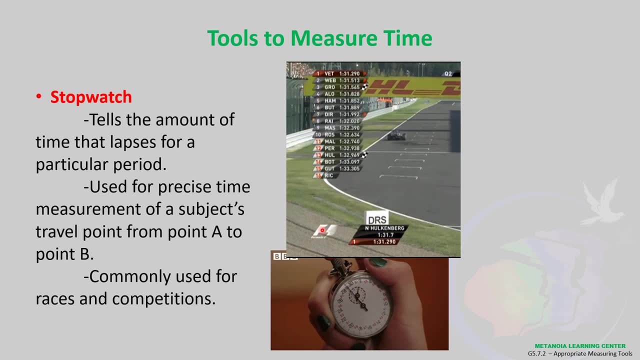 commonly used for races and competitions. if you notice, if you have watched, passed through a channel, for example, F1 Formula 1 race, if you see, this time this is actually their difference. split second, millisecond. that's the difference from the 1st to the 15th.